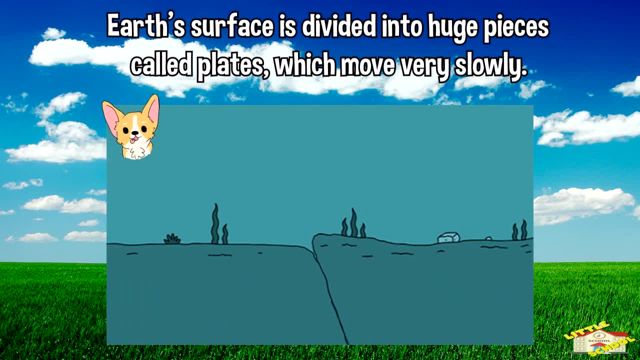 The theory called plate tectonics explains this type of mountain building. The theory called plate tectonics explains this type of mountain building. The theory called plate tectonics explains this type of mountain building. Earth's surface is divided into huge pieces called plates, which move very slowly. 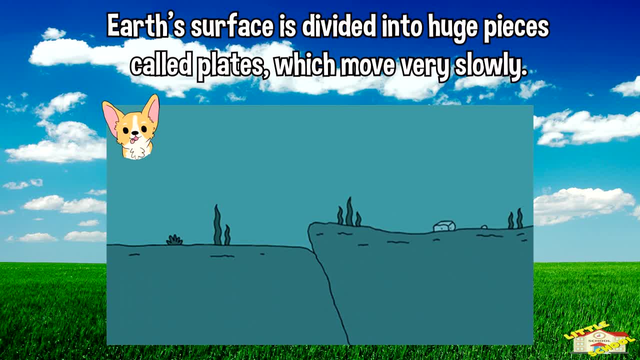 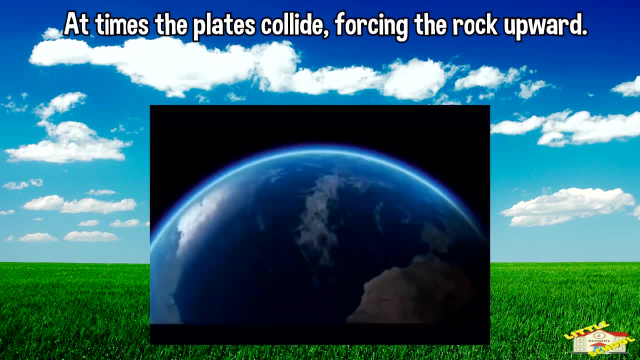 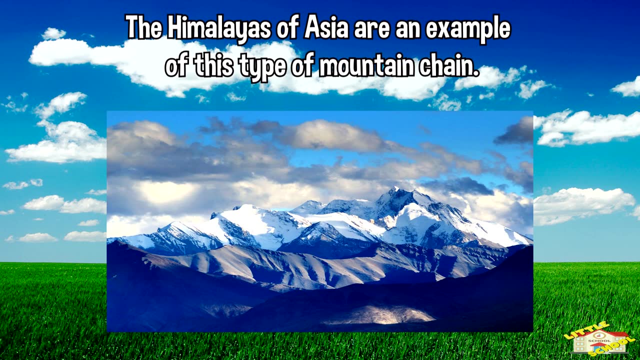 Earth's surface is divided into huge pieces called plates, which move very slowly. Earth's surface is divided into huge pieces called plates, which move very slowly. The continents sit on top of the plates and move with them. Earth's surface is divided into huge pieces called plates, which move very slowly. 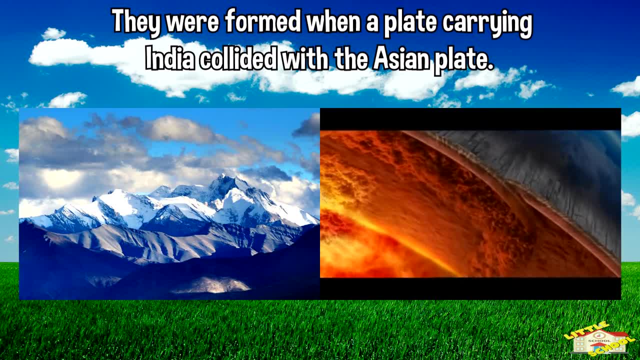 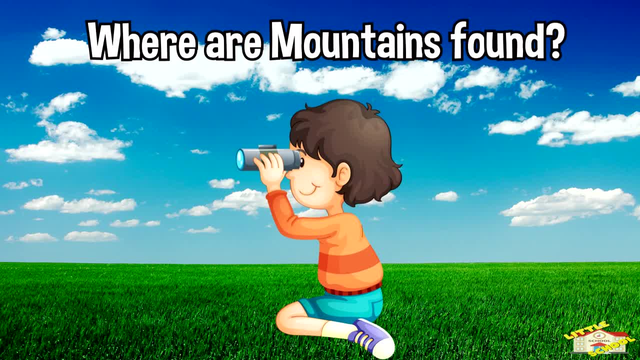 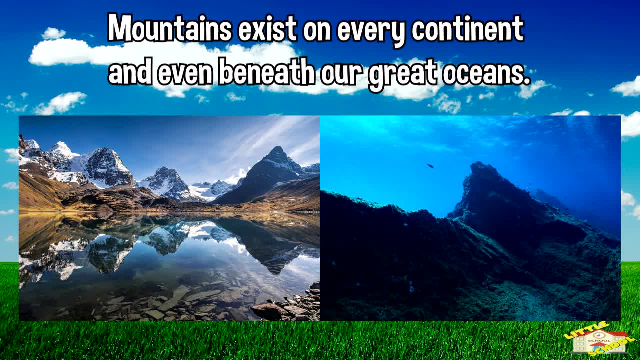 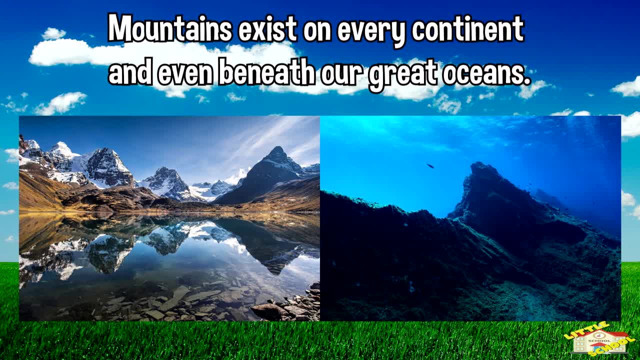 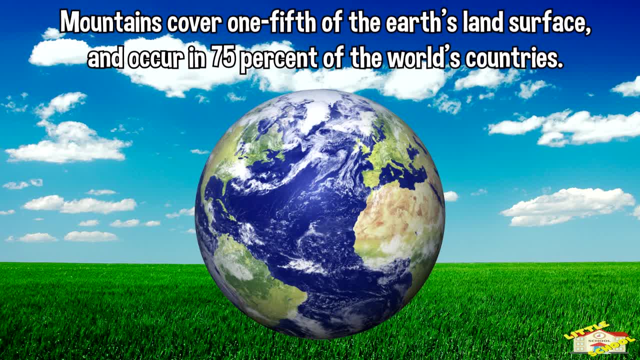 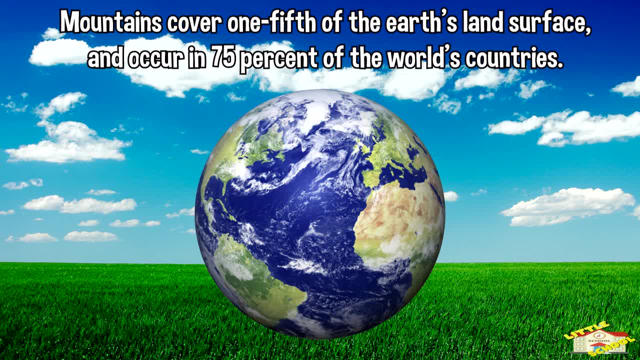 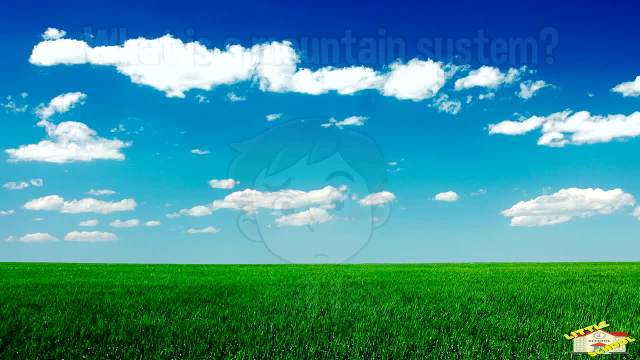 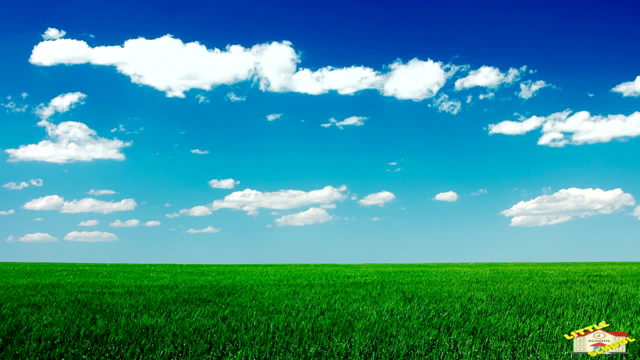 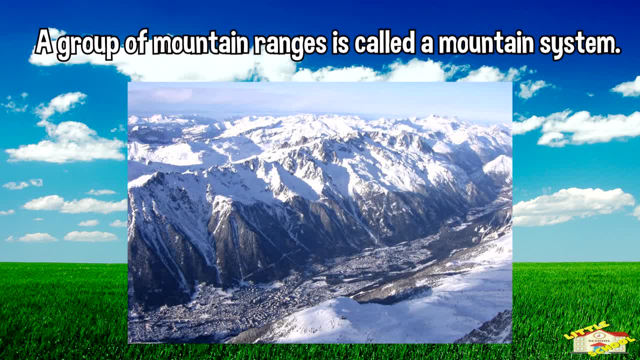 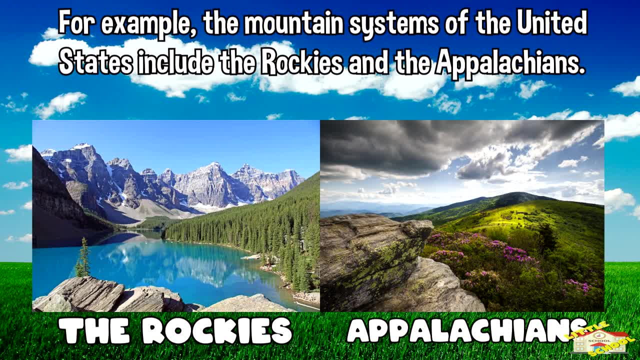 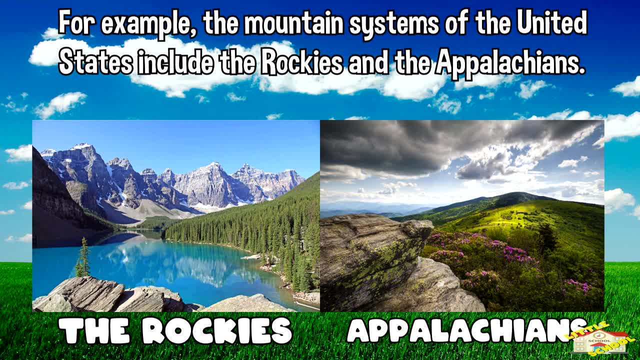 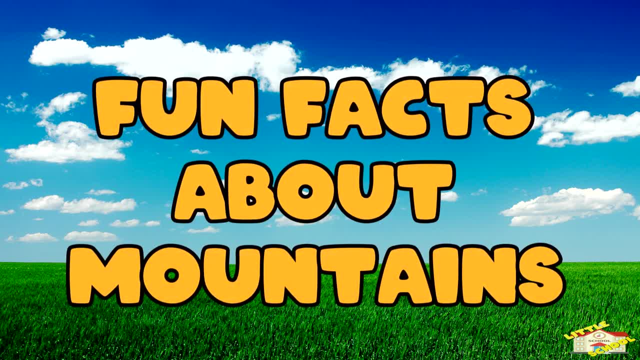 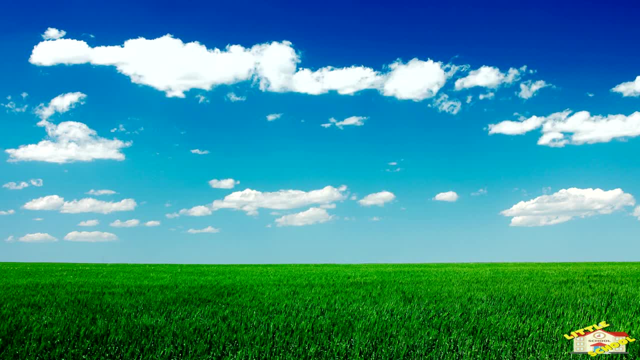 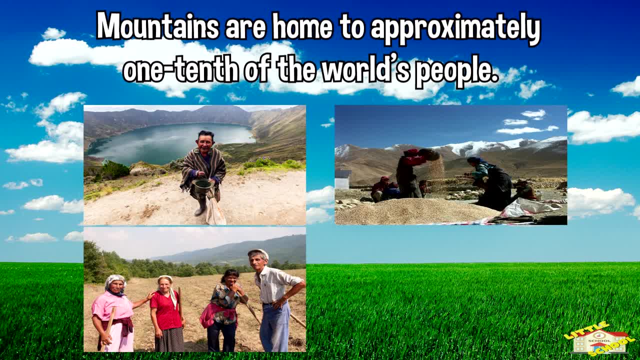 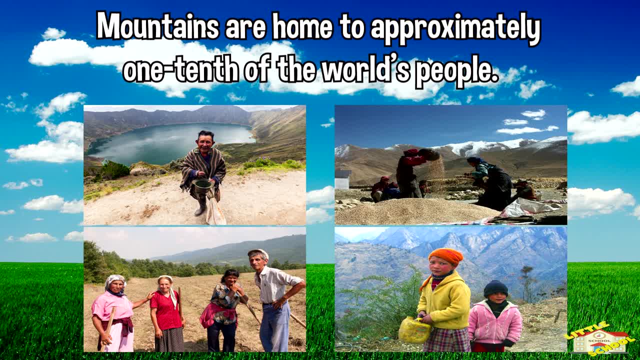 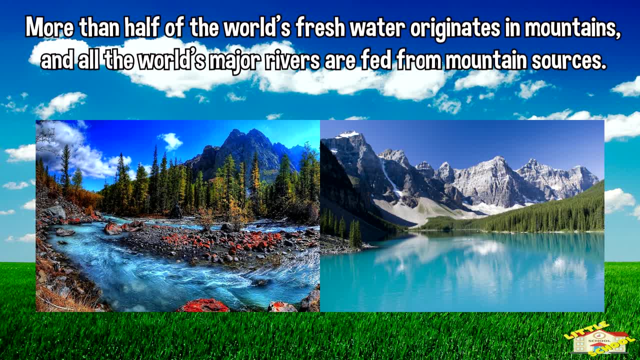 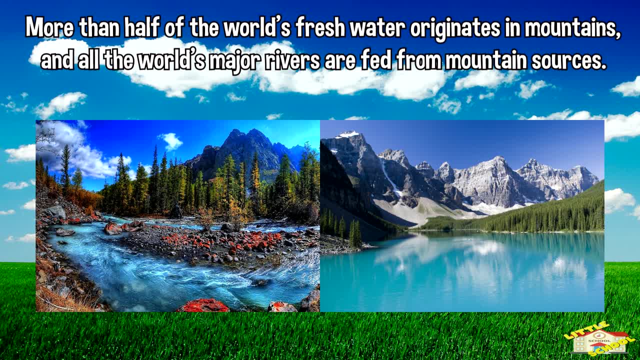 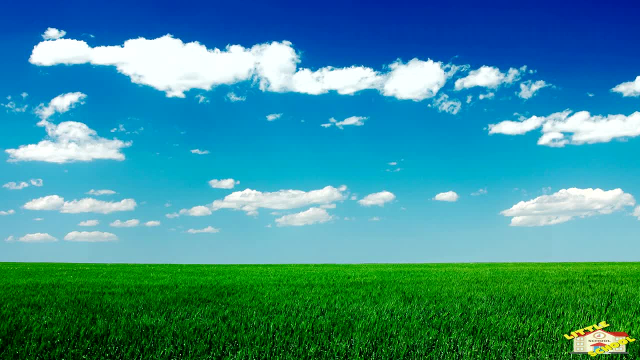 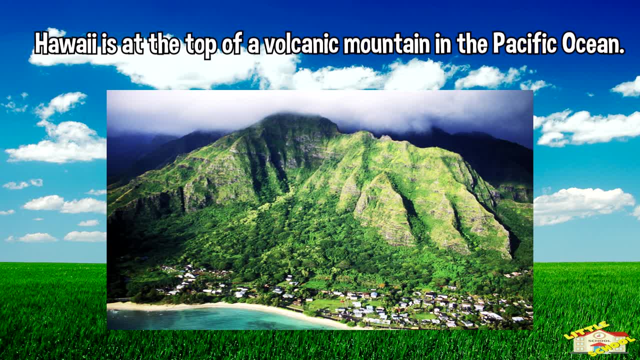 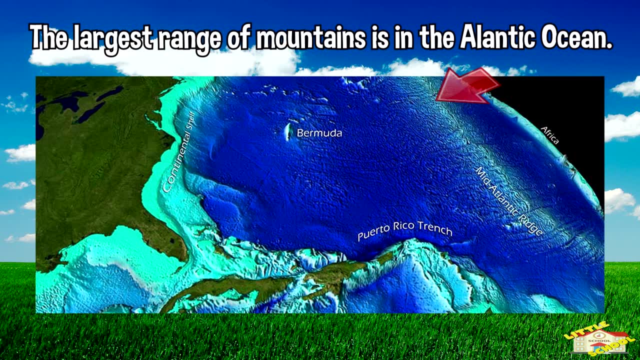 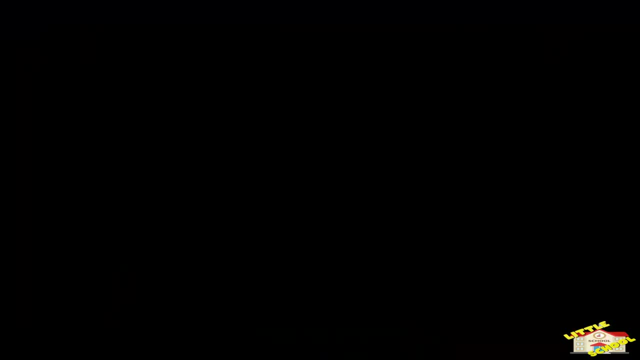 Hawaii is at the top of a volcanic mountain in the Pacific Ocean. More than half the mountain is below water. The largest range of mountains is in the Atlantic Ocean, And that is all for today's video. I hope you enjoyed learning about mountains today. 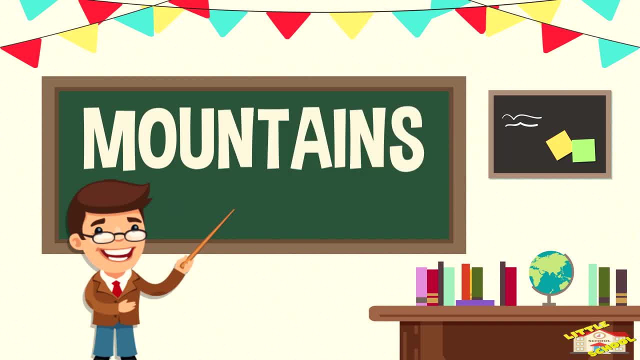 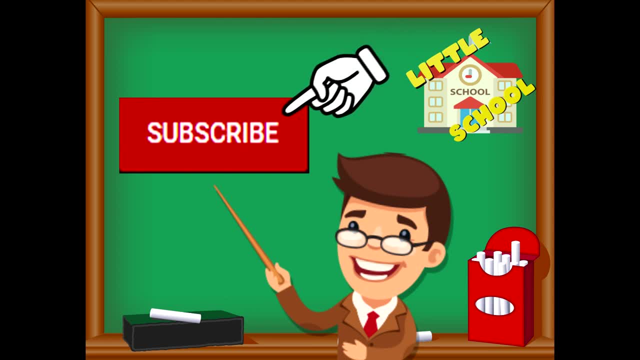 Take care now, Bye-bye. If you enjoyed the video and want to see more videos from us, please click the subscribe button. Also, give us a like. That will help us. We thank you so much and we do hope that you enjoy our videos. See you soon. 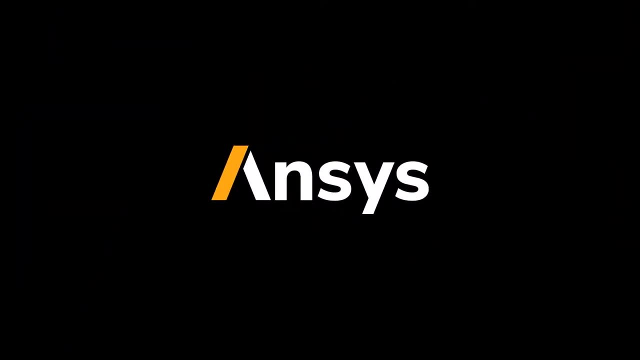 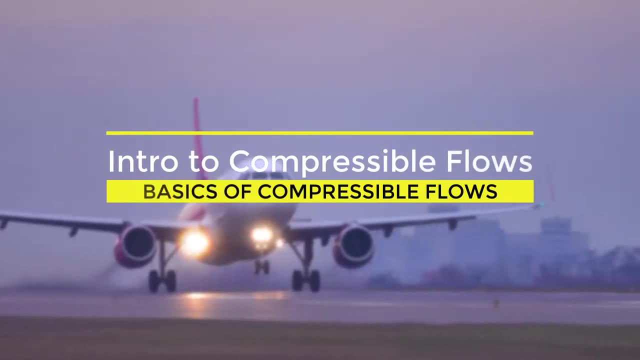 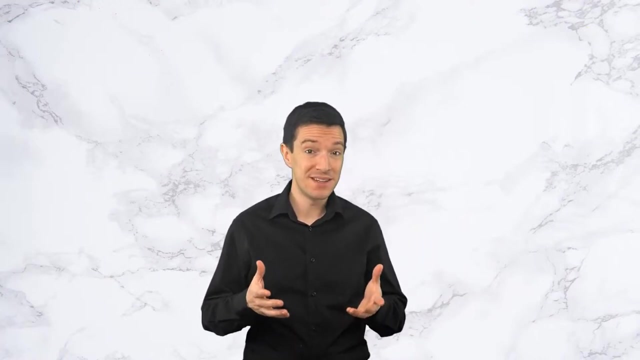 In this course, we will learn about compressibility and its importance. An incompressible fluid flow is defined as a flow where the density is assumed to be constant. In reality, no fluid is truly incompressible. In general, if the density variation in a flow is greater.